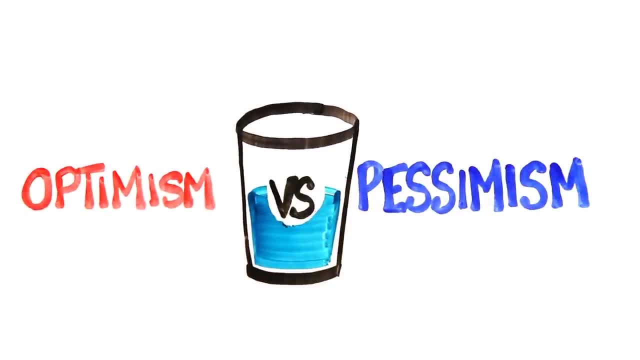 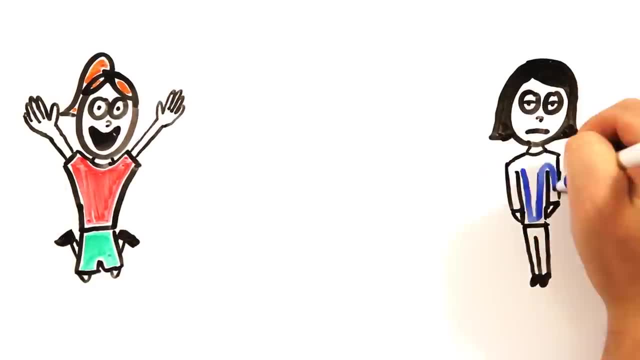 But in all seriousness, can science explain your emotional perspective and outlook on life? It turns out it may not be in your control. Research has shown that those with too long alleles on specific genes controlling for serotonin are more likely to focus on positive images, like someone enjoying ice cream. 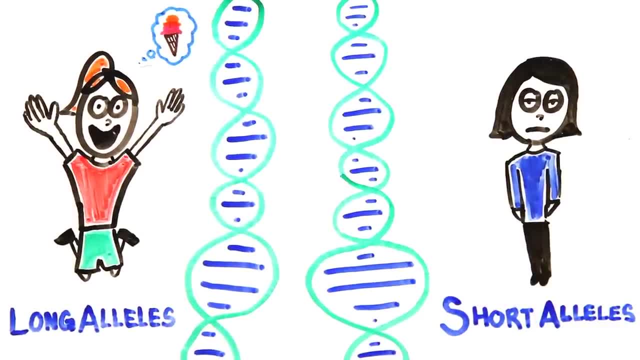 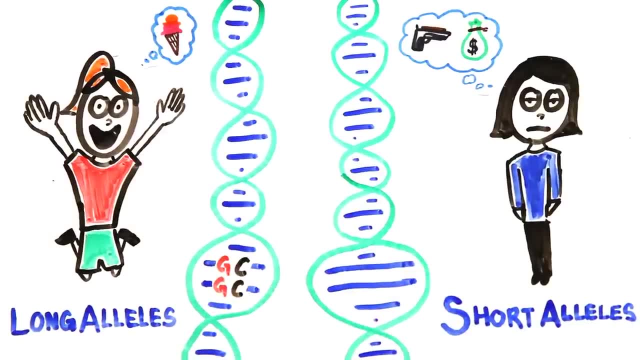 compared to those with a short allele on the same gene, who are more likely to focus on negative images, like someone being robbed. Variation in the oxytocin receptor gene can also affect your outlook. Individuals with two copies of guanine are noted to be more optimistic, with higher self-esteem. 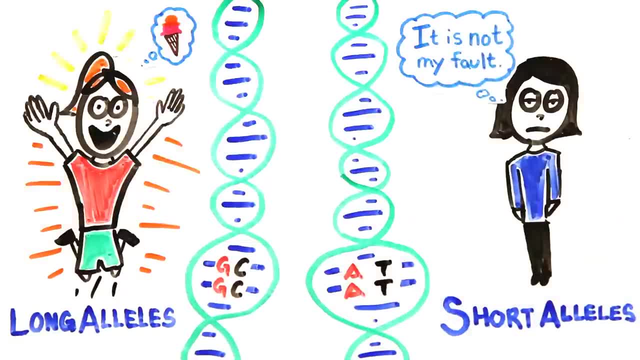 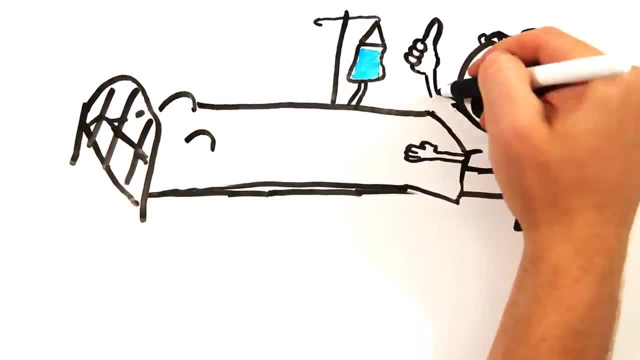 while those with copies of adenine were less positive. So it seems that people may be genetically susceptible to pessimism. Interestingly, optimists are less likely to be re-hospitalized after coronary artery bypass surgery, show higher academic achievements and even better socioeconomic status. 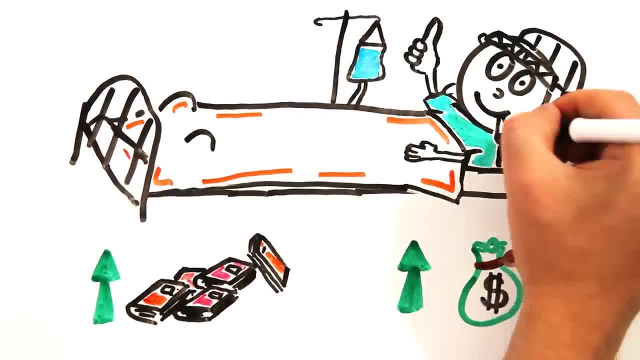 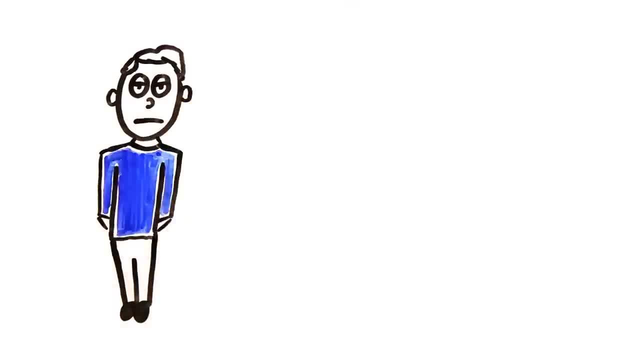 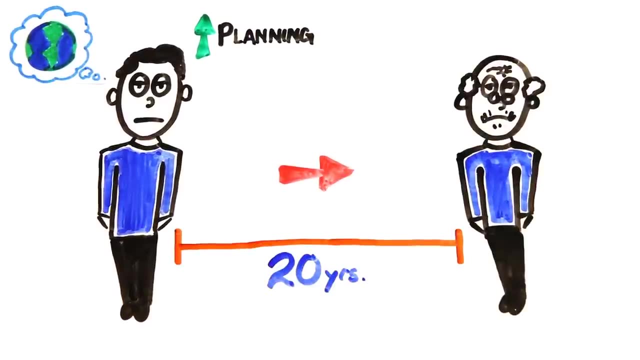 But it's not all good. They can overestimate their abilities and underestimate risk. Pessimists, on the other hand, have a more realistic view of the world, are more cautious when planning for the future and may even live longer. A landmark study spanning 20 years found that pessimists use a cautious approach to their findings. 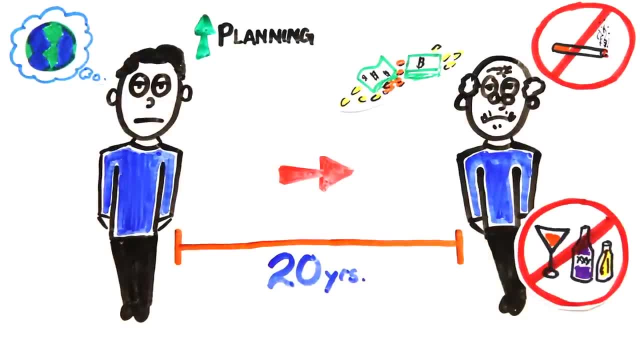 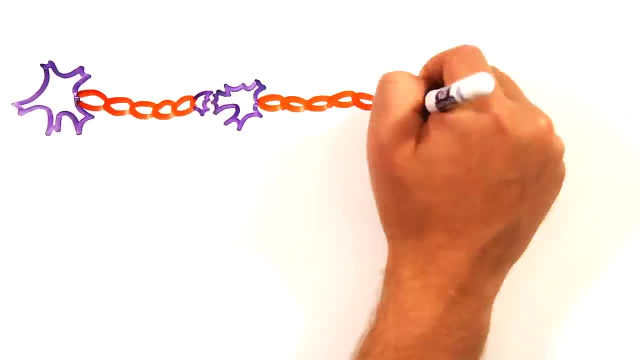 to improve their finances and health, avoiding risky behaviors such as smoking and excessive drinking, ultimately giving them the last laugh, Literally over-optimists, But statistically, most of us are hard-wired to lean towards optimism, Known as the optimism bias. 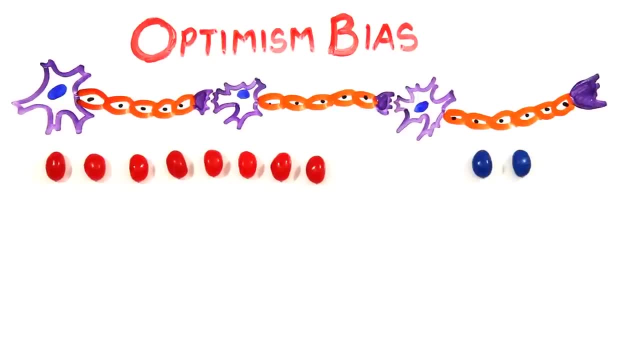 and found in around 80% of the population. we tend to overestimate the probability of positive events occurring in the future, while grossly underestimating the probability of negative ones, For example, even though the divorce rate can be as high as 40%. 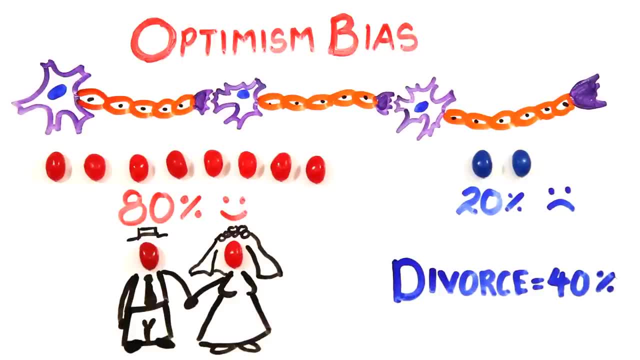 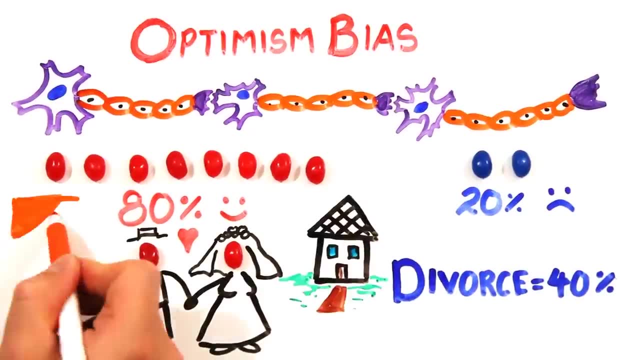 most newlyweds predict their probability of divorce to be 50%. The probability of getting divorced at 0% Chances are. when you imagine your future, it's usually better than your current situation. Furthermore, we often imagine ourselves as being more intelligent, sociable and honest than other people. 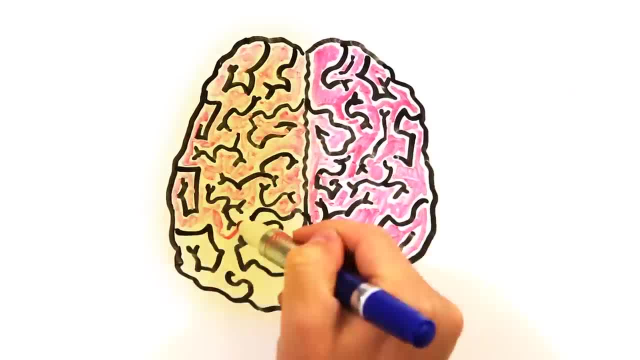 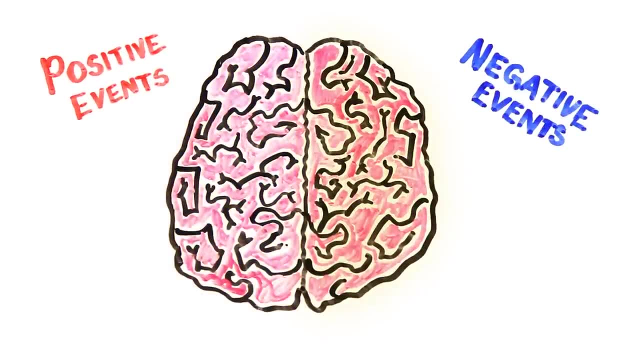 When we look at the brain, we actually see the left half exhibits increased activity when imagining positive events, whereas during negative events, the right half's activity does increase, but to a much lesser degree. This suggests that the brain chooses to ignore and filter out negative information.